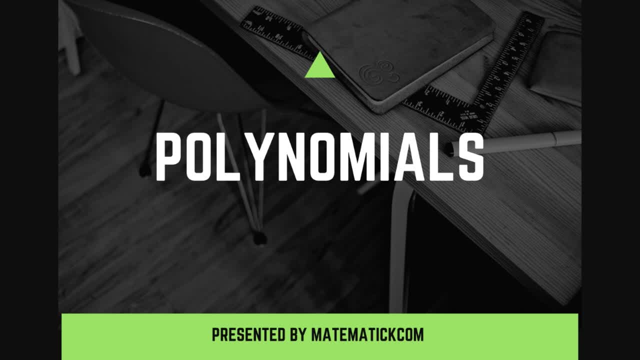 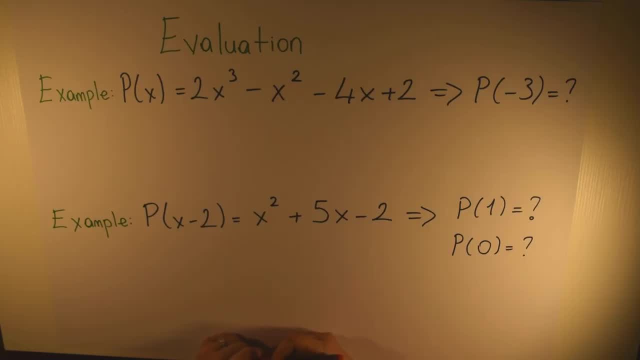 Now we will continue with the evaluation. So evaluation is a very easy process. You just take the value or values you have been giving, plug them in for the appropriate variables and simplify to find the result. So for example here we have: px is equal to 2x to the power of 3. 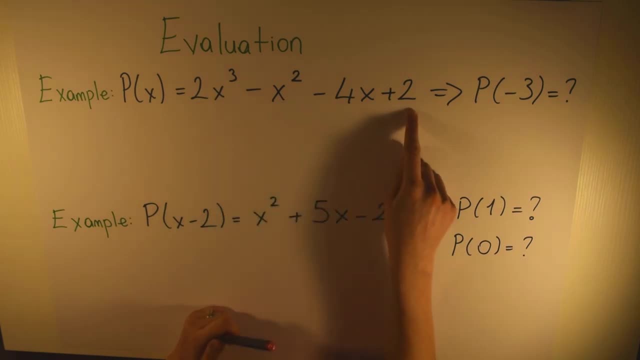 minus x to the power of 2 minus 4x plus 2 and p minus 3 is x. So what we are going to do? we are going to just put minus 3 instead of x here. So let's write them down Here we have 2 x to the 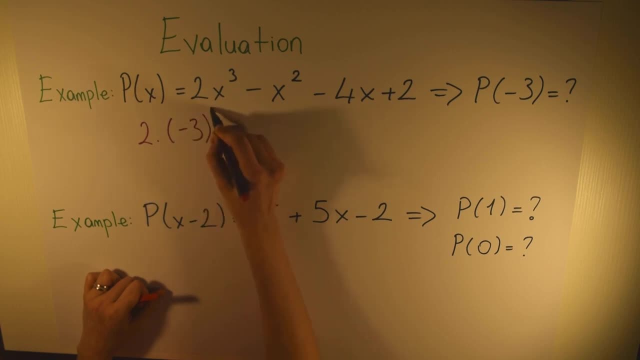 power of 3, which means minus 3 to the power of 3 minus x, to the power of 2, which means minus 3 to the power of 2 minus 4x. We write here: minus 3 plus 2 and then we have: this is minus 27 minus 27. 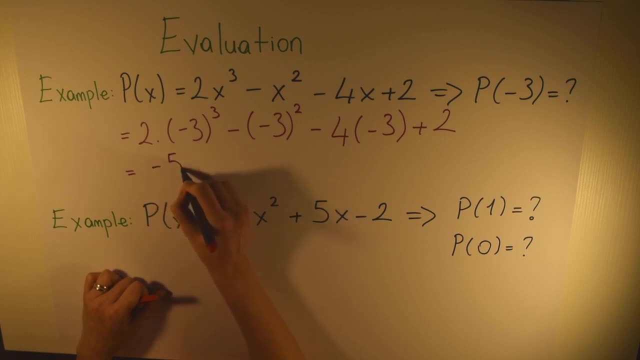 times 2 is equal to minus 54.. We have here 9, but we have here minus, so it makes minus 9.. Here we have plus 12 and we have here minus 9.. So we have minus 9 and we have here minus 9.. So we have. 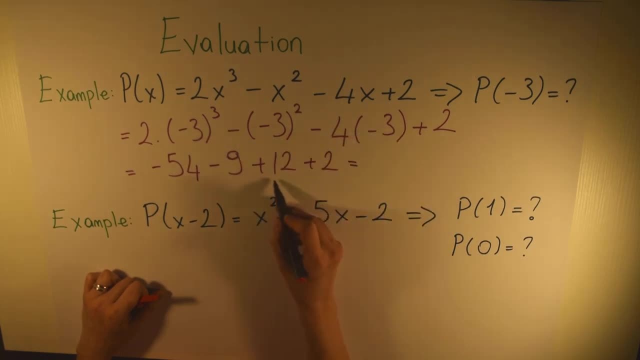 here plus 2. What we get from here? we have plus 14.. This makes plus 14.. This makes minus 40. and if this is equal to minus 49. You just put this value instead of x here. That's all you have to. 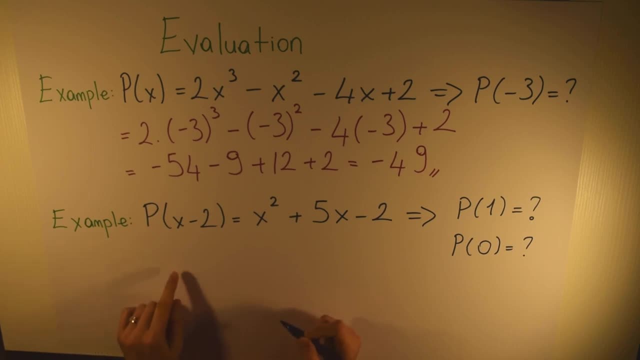 do. Let's look at our second example. Here we have: px minus 2 is equal to x, to the power of 2 plus 5x, and p1 and p0. they are asked So what we are going to do here to make this, to find p1. okay. 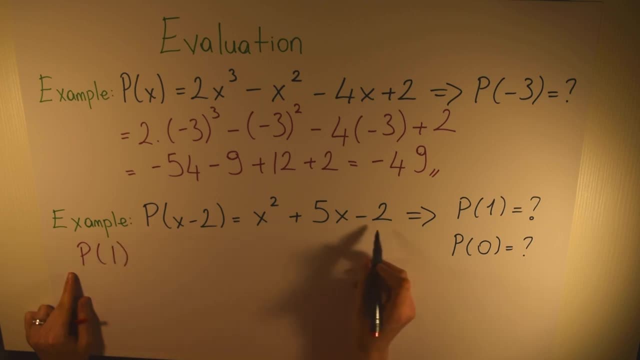 first we look at this original polynomial. Here we have x minus 2 right, So we will try to make this is equal to 1.. So instead of x, what, if, what should I put? here I should put 3 right, Because 3 minus 2 makes 1.. So which means here, instead of x, I will put. 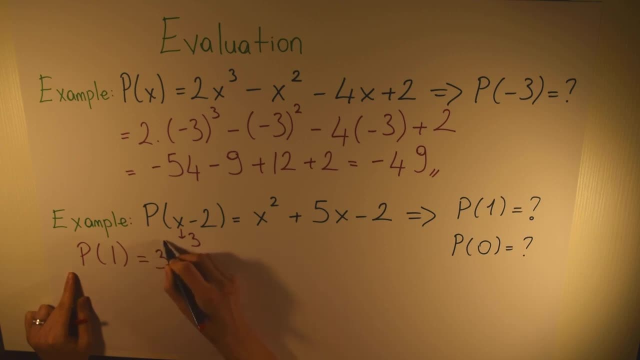 3.. So here we have 3 to the power of 2 plus 5 times 3 minus 2.. And here we get 9 plus 15 minus 2 and we get 21.. 2 from here, and the second one is the same, to find the p zero. okay, we look at here what makes. 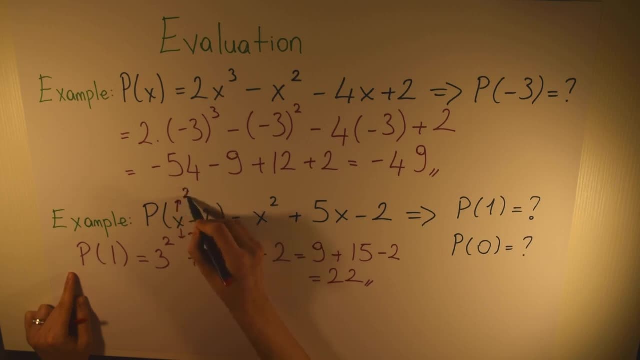 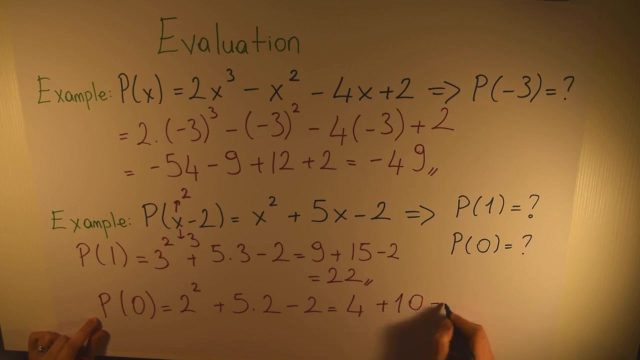 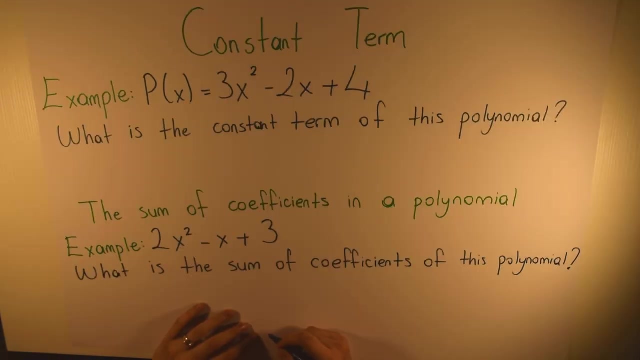 this zero. when we put 2 instead of x, we get p zero right. so we write here: p zero is equal to: we put here 2 to the power of 2 plus 5 times 2 minus 2, this is equal to 4 plus 10 and minus 2, which is equal to 14 minus 2- 12. now we will continue with the constant term. 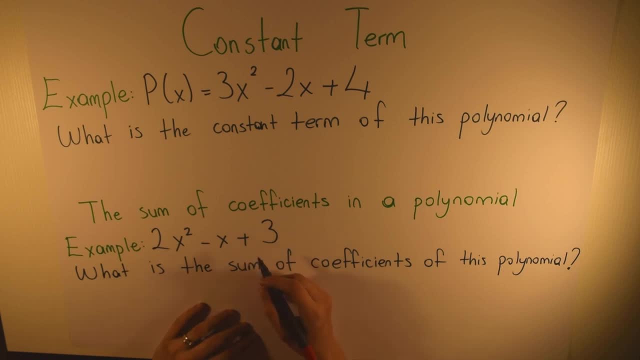 the constant term of a polynomial is the term of degree zero. it is the term in which the variable does not exist, the term in which the variable does not appear. so here, for example, we have p. x is equal to 3, x to the power of 2 minus 2, x plus 4. so it's asking: what is the, what is the constant term of this? 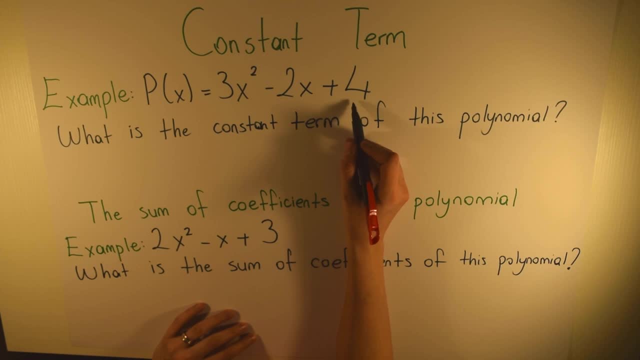 polynomial. we already actually know that here, 4 is our constant term, but sometimes you will see much complicated questions, so you will need to use this trick. what we do? instead of x here we write zero. okay, instead of x we write 0, which means we will find p0.. Let's look at this: here We have 3 times 0 to the power. 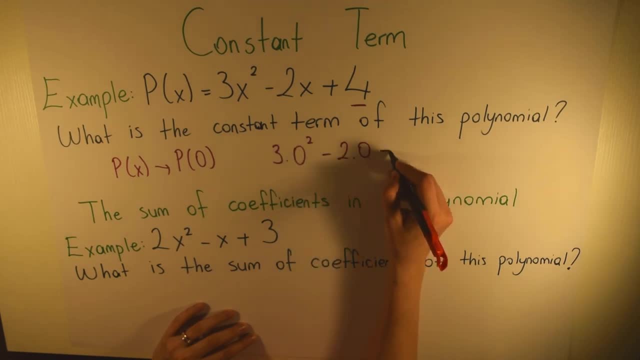 of 2 minus 2 times 0 plus 4.. So from here, these are 0, so we get 4.. Okay, you just need to destroy these terms with the variables. Okay, let's look at the sum of coefficients in a polynomial, So. 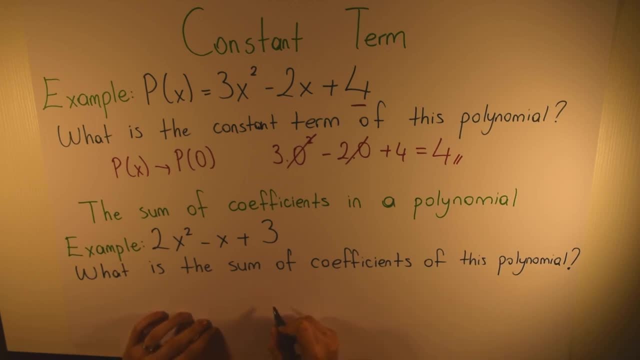 here what you should know, that you should find p1.. Okay, so instead of x, you write 1 and you will find the sum of coefficients. Let's look at this example: 2x to the power of 2 minus x plus 2.. 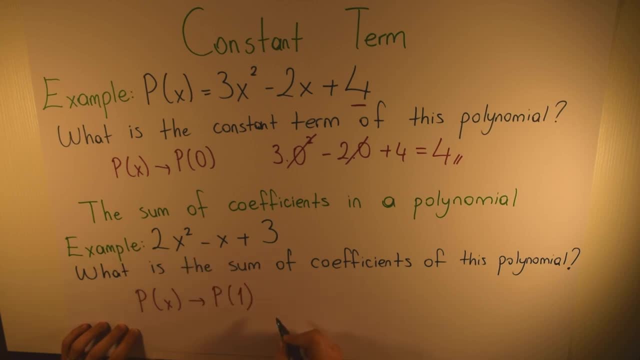 So how we find? We just write 1 instead of x. Okay, so we write here: p1 is equal to 2 times 1 squared minus 1 plus 3.. We have here 2.. We have minus 1, 1 plus 3.. We get 4.. Also, without using these three, we can also: 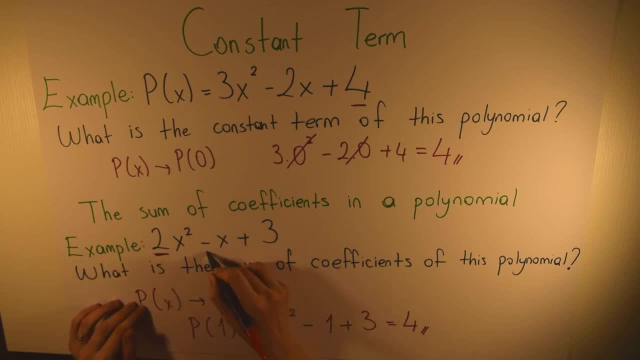 find the sum of coefficients. Let's look at: We have 2 here, We have minus 1,, 2 minus 1.. We get 1 plus 3.. We get 4.. Same thing, But, as I said before, like here, sometimes we can see much complicated. 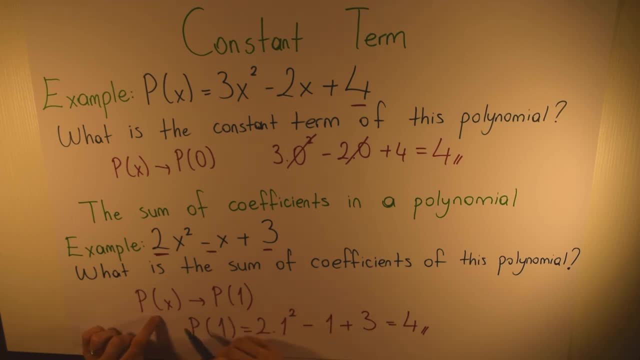 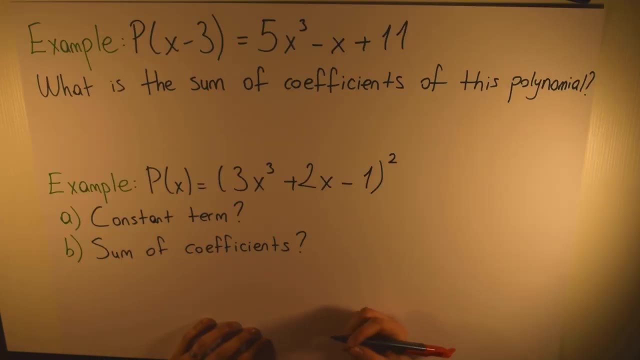 questions. In those questions we should use this trick. Let's continue with other examples. So here we have: px minus 3 is equal to 5x, to the power of 3 minus x plus 11.. What is the sum of coefficients? 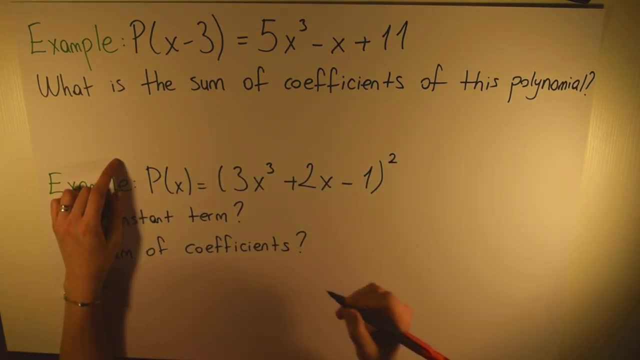 of this polynomial. Well, remember, this is the Furthermore part. So, as you can see in the previous example, you can see all these coefficients. Well, we write here p to the power of 3 minus 1, squared minus 2 squared minus 1 plus 3.. So let's just write it again, Okay, If you already? 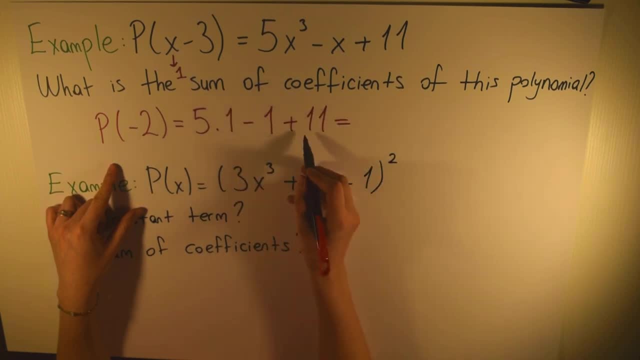 understood the problem. remember to write this here. We have an interval. Now we have a interval, So the interval is equal to 1 times 1 squared minus 1, plus 11 squared minus. So our answer is 15.. It is also obvious here: 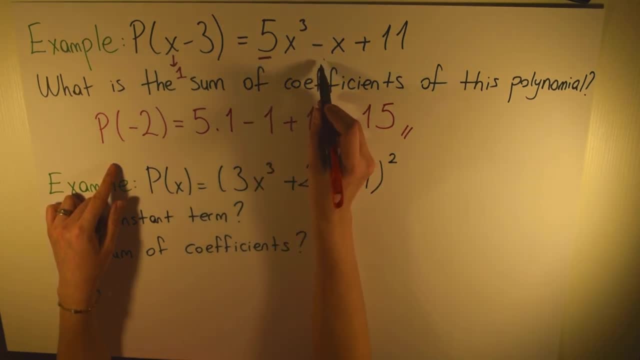 Here 5. we have minus 1. we have here It's 4 plus 11.. It is equal to 15, the same answer. Let's look at this example: Px is equal to 3x to the power of 3 plus 2x minus 1d is all to the power of 2.. 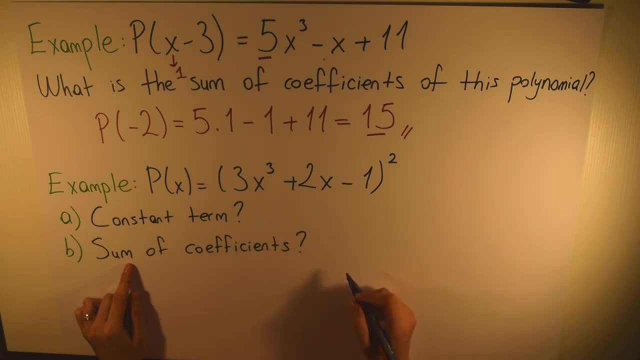 Okay, if we extend this polynomial by taking a square of it, it will be too long. So what we do? we use our tricks, So to find the constant term, what we should do, we should put 0 instead of x. 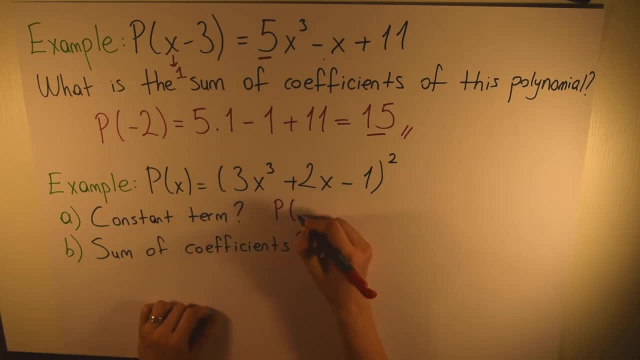 So we should find P0. here, Sum of coefficients is the same. What we should do, we should put 1 instead of x, So we should find P1.. Okay, let's find P1.. Let's find P1.. Let's find this. 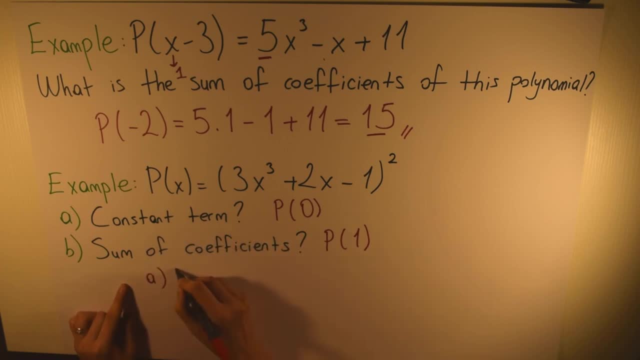 So the first one, P0, is equal to 3 times 0 plus 2 times 0 minus 1 to the power of 2.. These are 0 minus 1 and we get here 1. And here we should find P1, right. 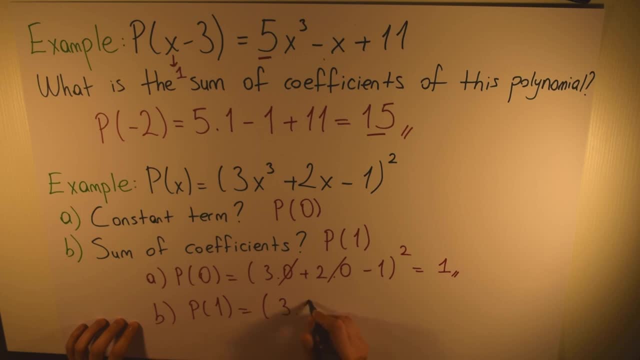 So we have here 3 times 1.. 1 plus 2 times 1, because this is 1 to the power of 3.. It's 1. And minus 1 to the power of 2. This is 3, 5, minus 1.. 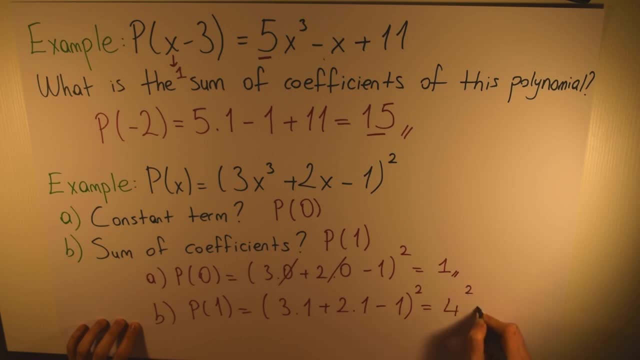 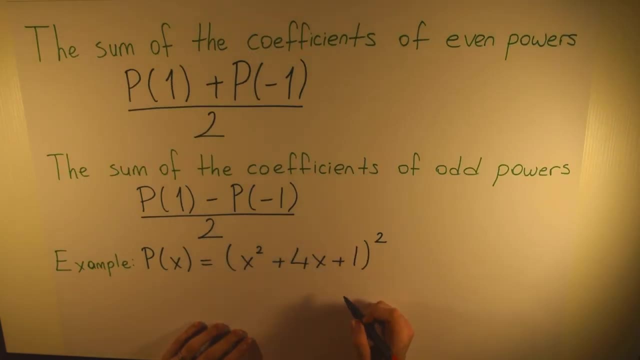 It's 4.. So the answer is 4 squared, which is equal to 60.. Let's continue with the sum of the coefficients of even powers and odd powers. So we have specific formulas For this. for example, when we have a polynomial and it has powers like x to the power of 2,. 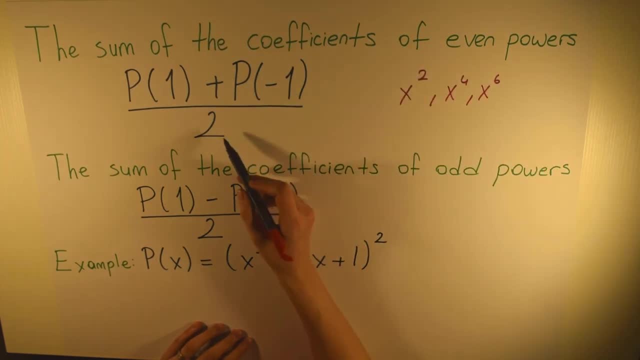 x to the power of 4, x to the power of 6, we use this formula: Instead of x, we write 1 and we find P1 plus P minus 1 over by 2.. Okay, this is a specific formula for this.